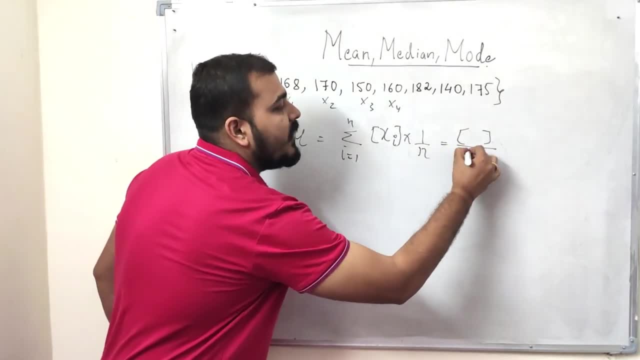 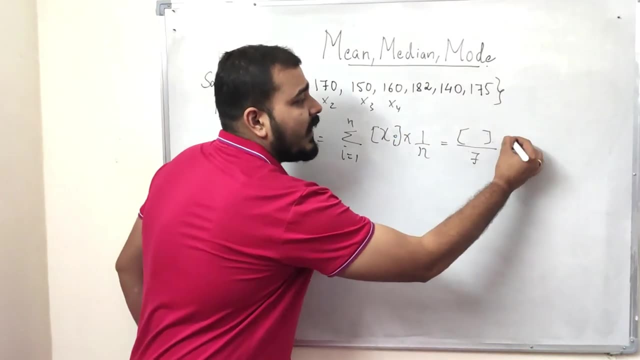 add up this and I'll then finally, whatever will be the total count, I will divide by n. n is basically my values, that is 7.. Okay, which is the total count of the sample distribution. Now, after that, I will be getting a value as 63.5.. Suppose this is the output and the mean that I have basically got. 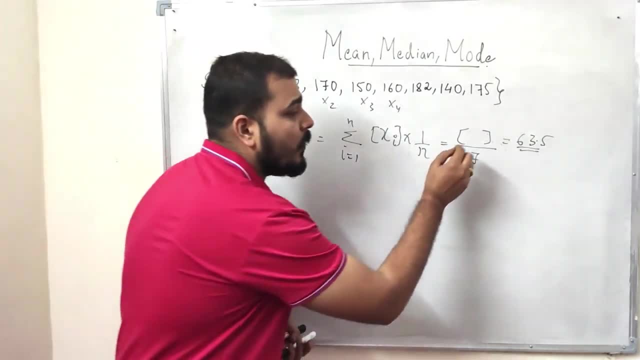 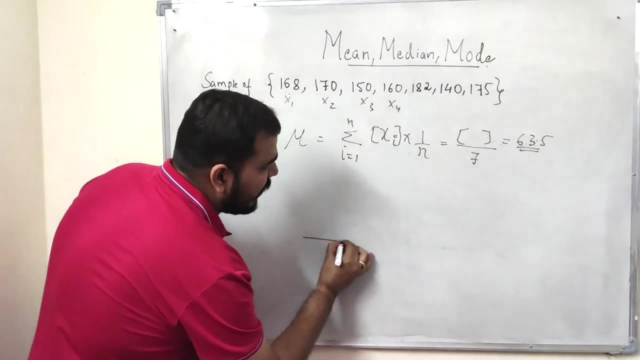 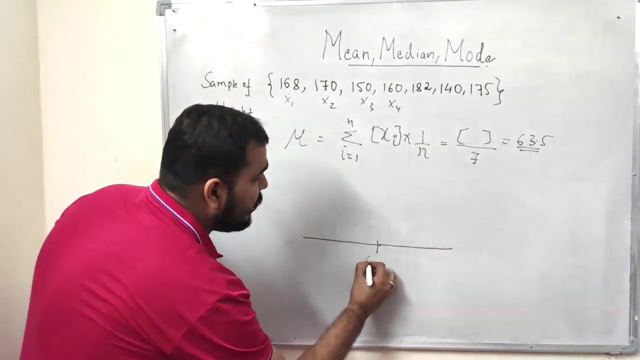 which is like 63.5.. Now let me specify some important properties about the 63.5.. Now, as you know that this is a sample of distribution of ages, So in your sample of distribution of ages, this 63.5 is the measure of central tendency. that basically means most of. 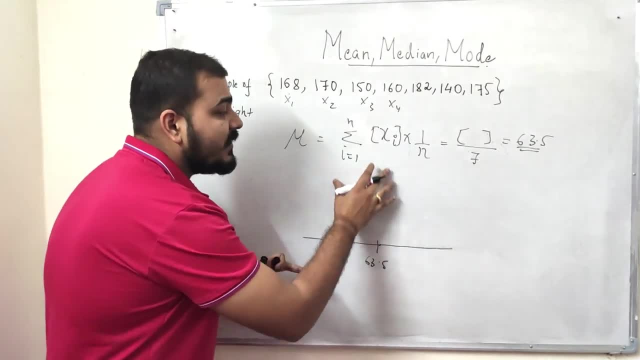 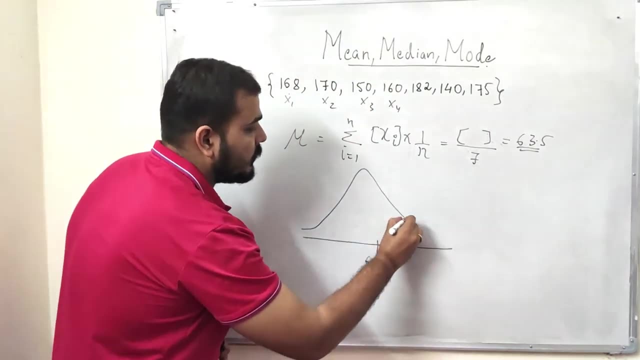 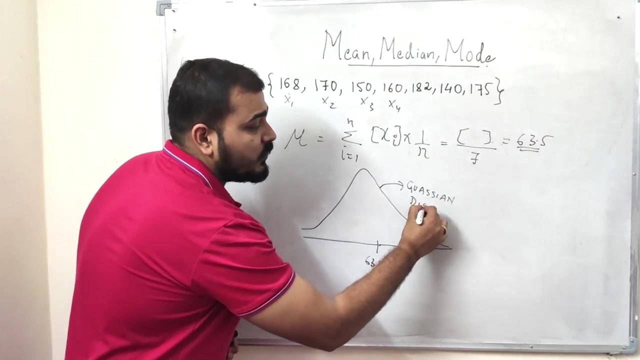 your edge, most of your age will be falling in this particular region. and suppose, if you increase some number of distribution of sample, you will be getting a curve which looks like this and this is basically your Gaussian distribution. again, I'll be explaining you about this in our future classes, but 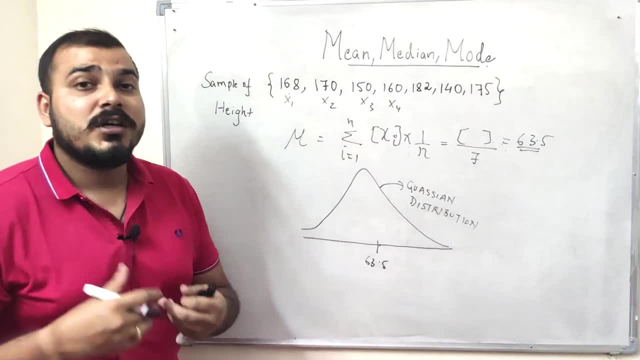 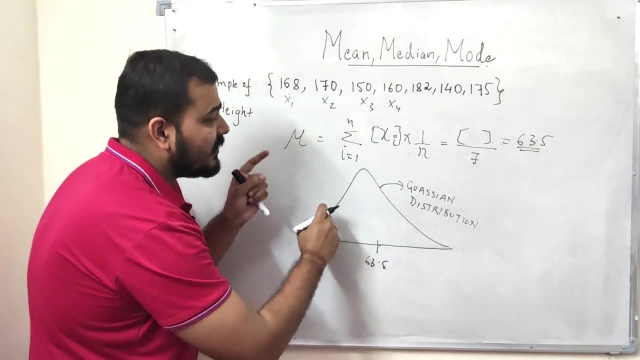 just understand. this is basically my Gaussian distribution and I can also term it as normal distribution, okay, and the central tendency, because over here you can see that this region is little bit. you know, this is basically a bell curve. more amount of values will be present in this particular region and if 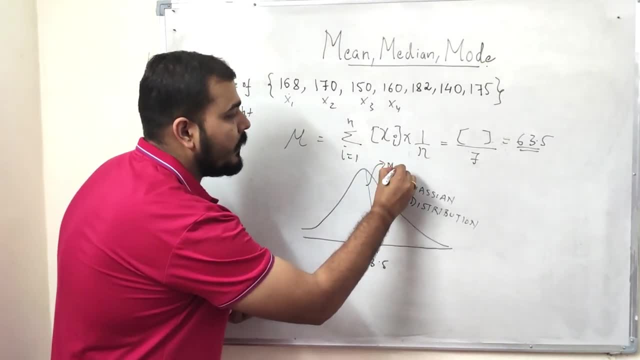 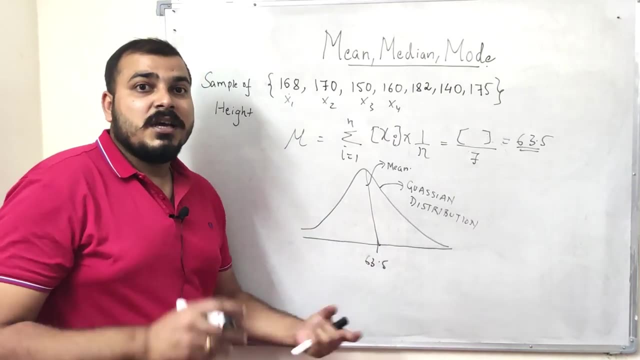 I just draw a line of this. this is basically my mean. okay. now this mean actually specifies the measure of central tendency. okay, so just understand this much. in the later upcoming videos I'll be explaining about variance, standard deviation and all also. so this is my mean, okay. 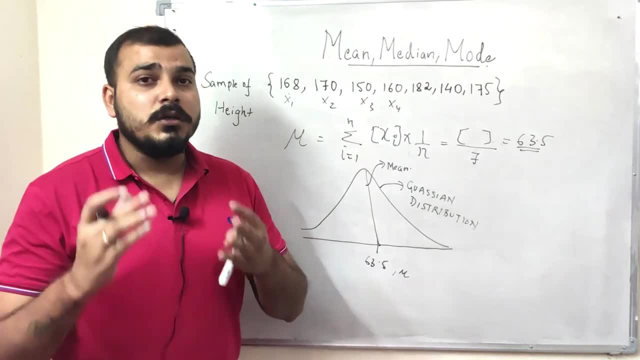 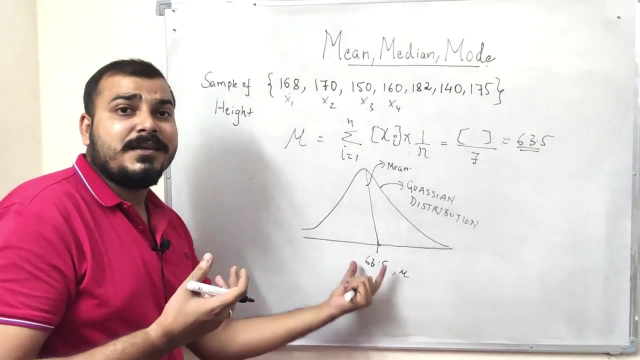 and now this is my mean. okay, so this is my mean. okay, now this is my mean, okay. mean can come into lot of use, which I'll be discussing in just a while, but just understand what does exactly mean? specified specifies the measure of central tendency. so let us just go ahead and try to understand why exactly median 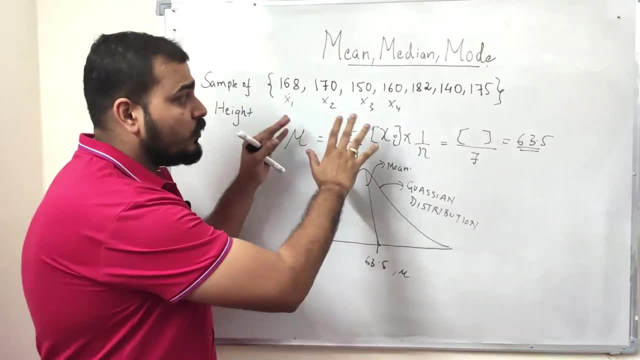 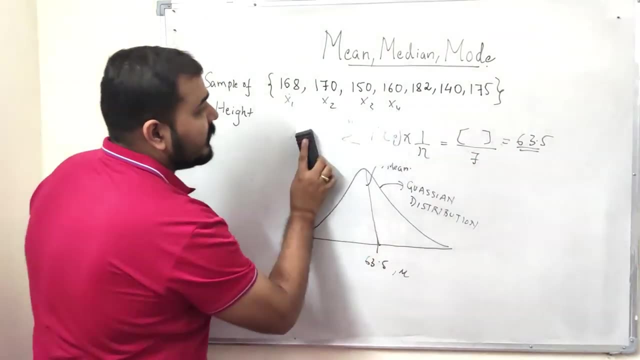 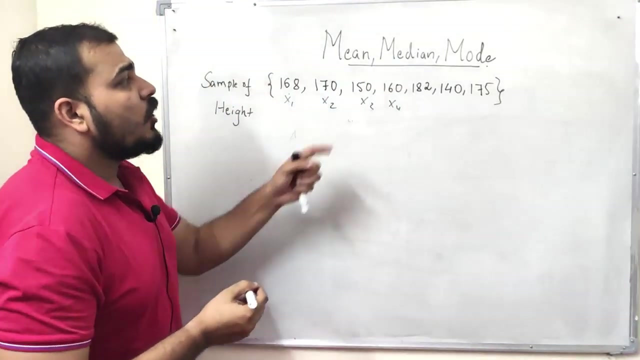 is also used. and finally, I'll also take a real world example and try to show you, to you, that how this mean can play a very good role. so let us just go ahead and try to understand what is exactly median. Okay, Now, in order to understand median, let us take a small example. I have a distribution like 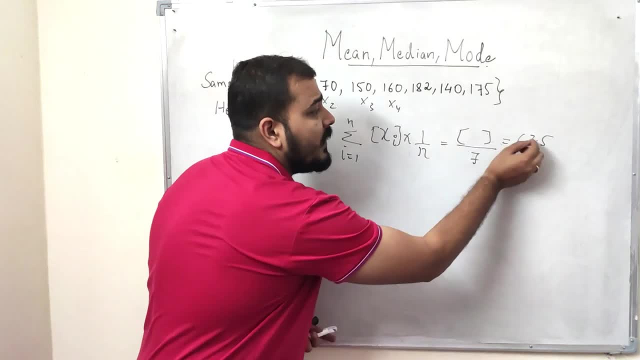 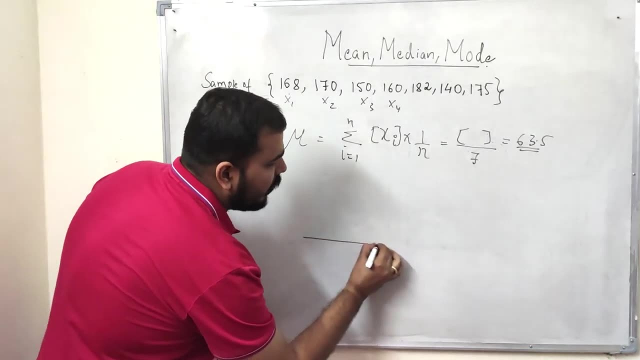 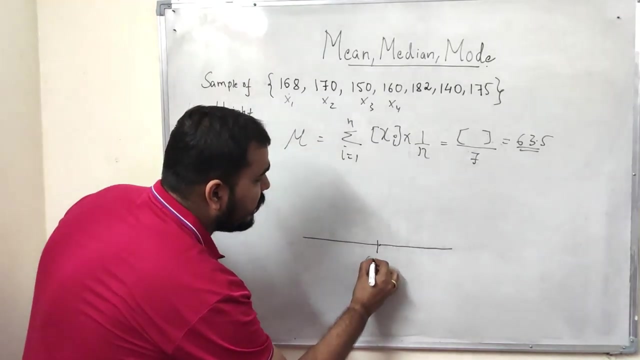 like 63.5.. Now let me specify some important properties about the 63.5.. Now, as you know that this is a sample of distribution of ages, So in your sample of distribution of ages, this 63.5 is the measure of central tendency. That basically means most of your, most of your age will be falling. 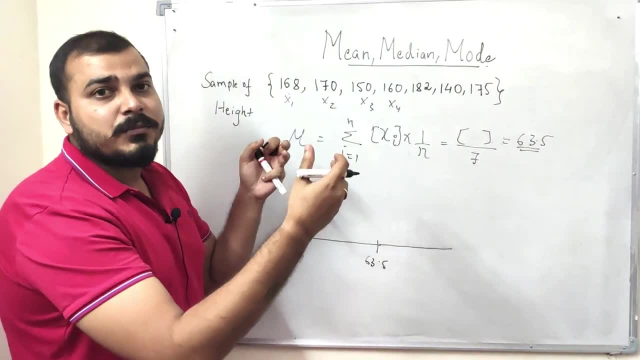 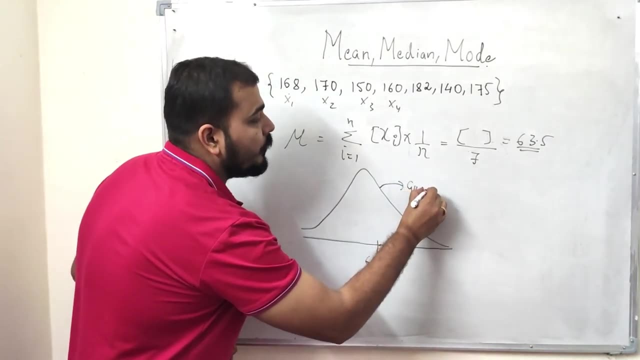 in this particular region And suppose, if you increase some number of distribution of sample, you will be getting a curve which looks like this, And this is basically your Gaussian distribution. Again, I'll be explaining you about this in our future classes, but just understand this is. 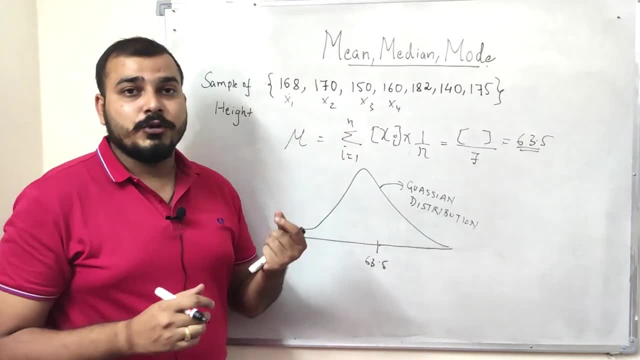 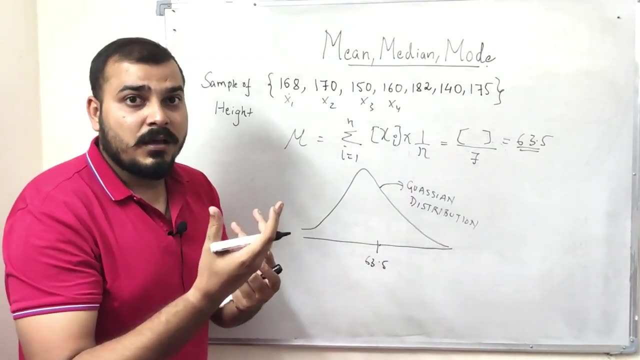 basically my Gaussian distribution- and I can also term it as normal distribution- And the central tendency, because over here you can see that this region is little bit. you know, this is basically a bell curve. More amount of values will be present in this particular region And if 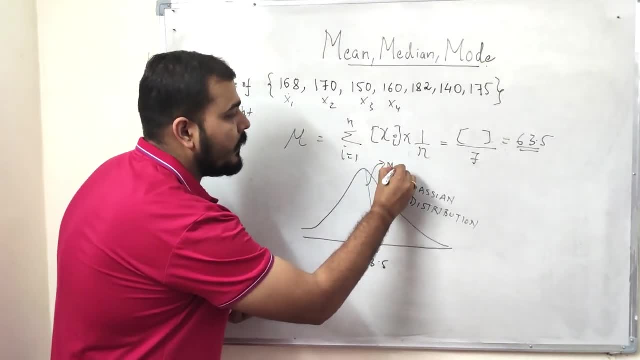 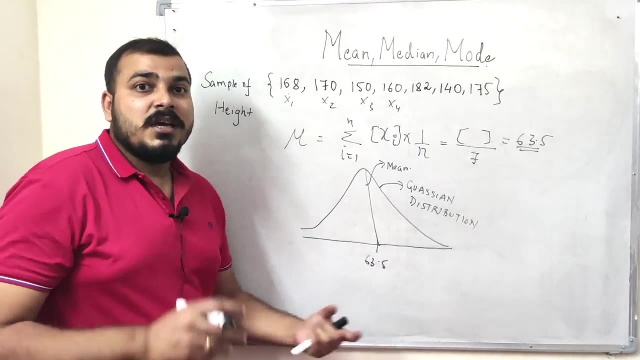 I just draw a line of this. this is basically my mean, Okay. Now this mean actually specifies the measure of central tendency. Okay, So just understand this much. in the later upcoming videos I'll be explaining about variance, standard deviation and all also. So this is my mean, Okay. 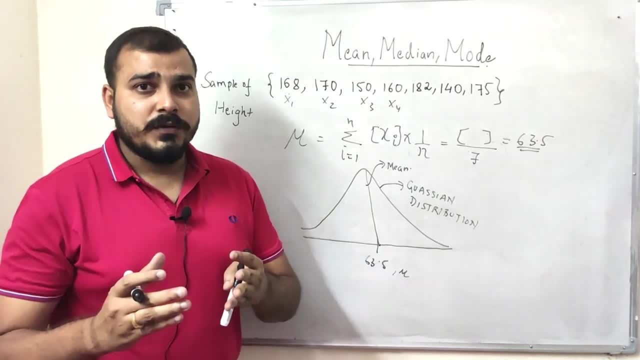 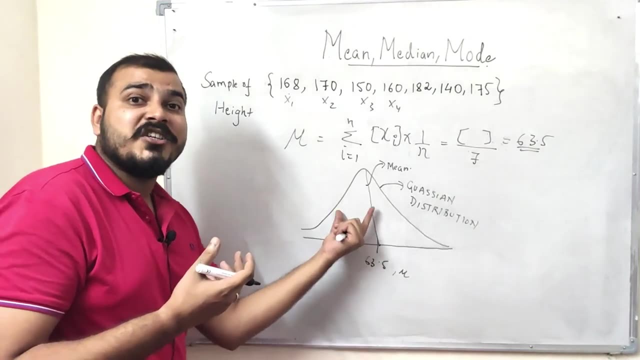 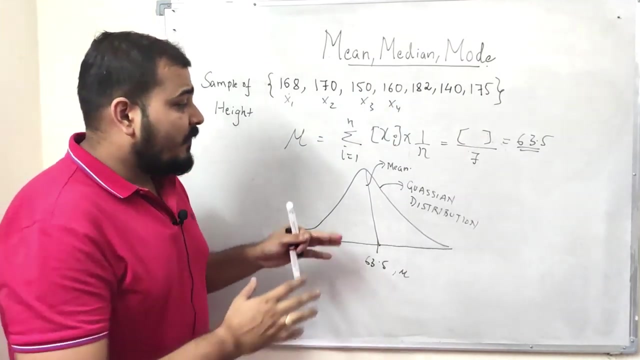 And now this mean can come into a lot of use, which I'll be discussing in just a while. But just understand what does exactly mean specified? specifies the measure of central tendency. So let us just go ahead and try to understand why exactly median is also used. And finally, I'll also take a real world example and 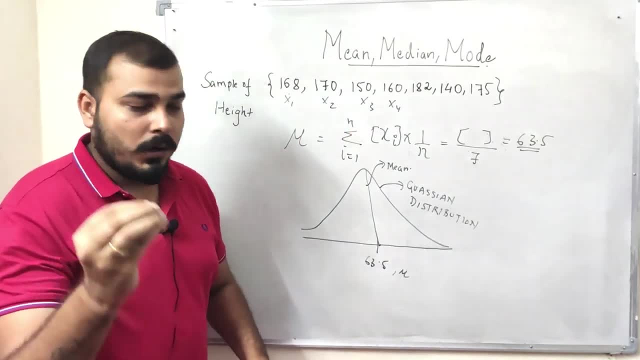 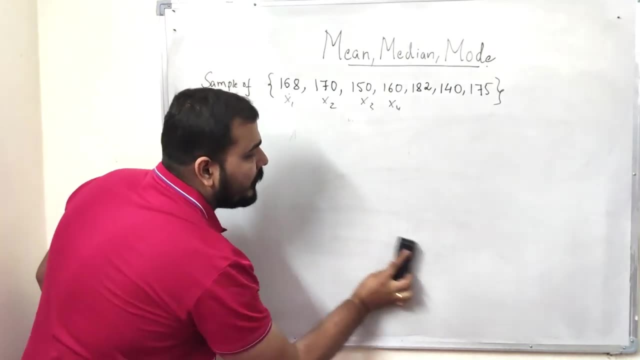 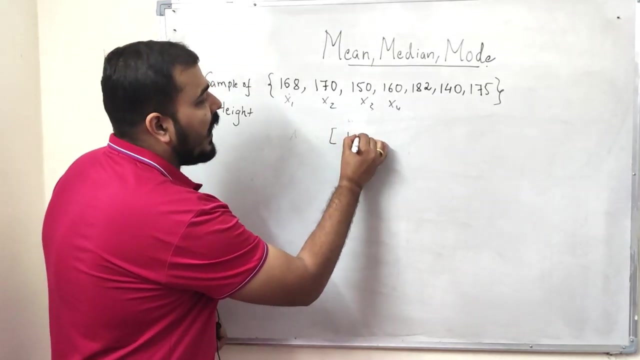 try to show you, to you, that how this mean can play a very good role. So let us just go ahead and try to understand what is exactly median. Okay, Now, in order to understand median, let us take a small example. I have a distribution like one, two. 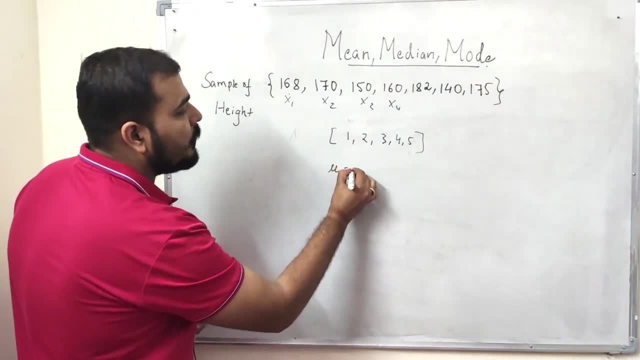 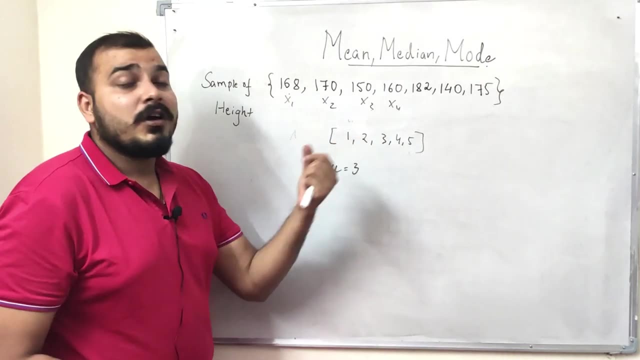 three, four, five And if I calculate the mean, the mean over here will be somewhere around three. It is just like you are adding up all this number and dividing by the total number of total count of this number. So this basically becomes 15 by 5.. Right, Because if I add it up, 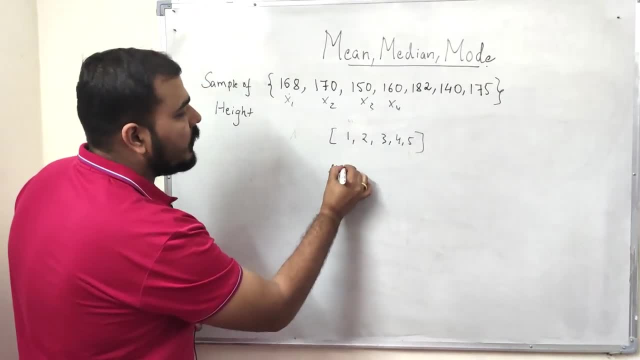 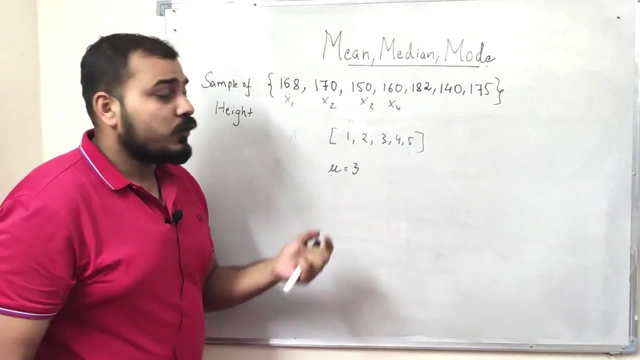 one, two, three, four, five And if I calculate the mean, the mean over here will be somewhere around three. It is just like you are adding up all this number and dividing by the total number, total count of this number. So this basically becomes 15 by five, right? Because if I add it, 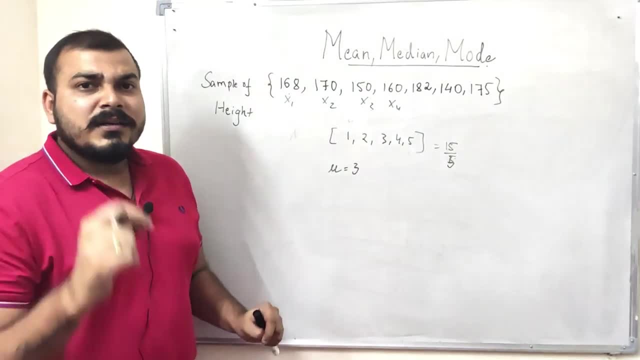 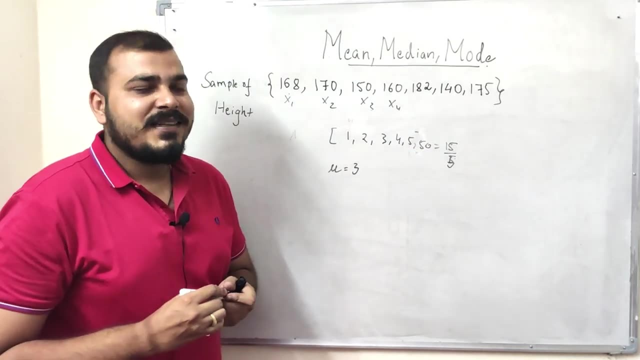 up it will be 15.. 15 by five is nothing but three. Now guess, just understand. if I add an outlier like 50, okay, this outlier basically specifies that this number will be a huge number. It will not be similar to this particular distribution. So suppose I have added 50. 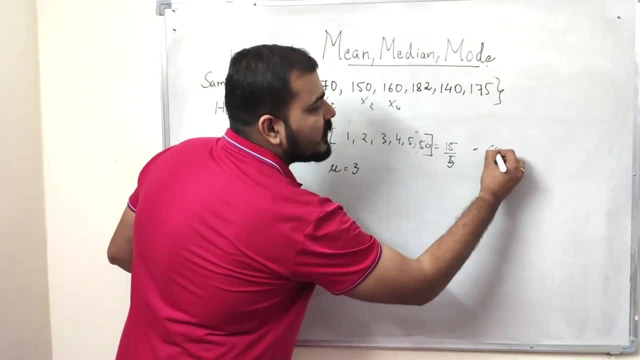 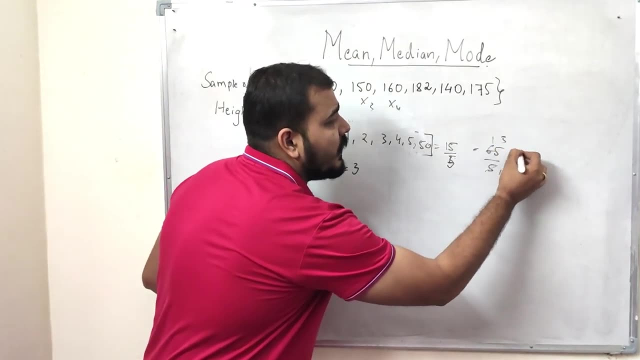 Now what will happen is that if I add this up, the total value will be 65 divided by five. right Now, if I try to see how much this is, five ones are three, So 13 is my value. that I'm. 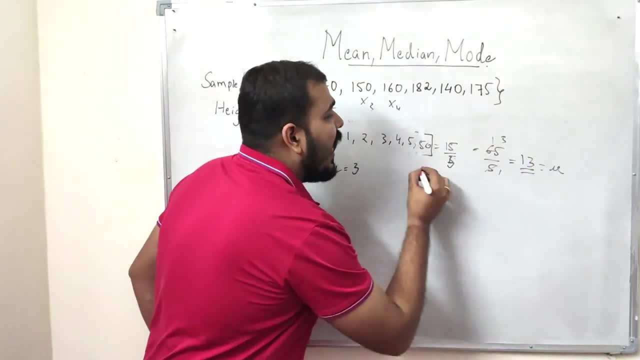 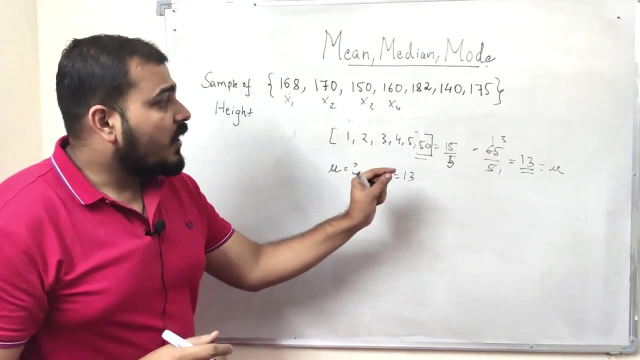 basically getting. Now understand, guys, this is my new mean after I added an outlier 50. Now you just see the difference of an outlier- sorry- difference of the mean, because I have added just an outlier. Now this basically represents a complete different format of. 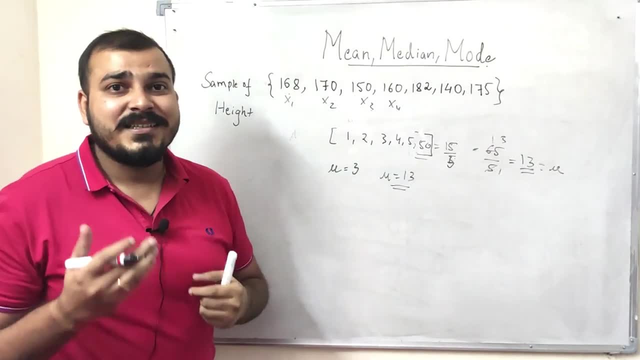 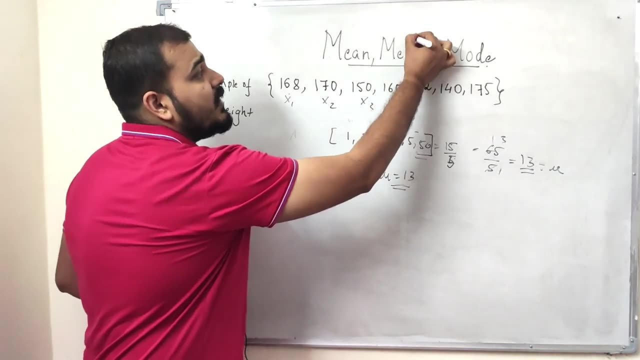 the distribution, And this is very, very harmful for doing any statistical analysis. So in this case, if I want to find out the central tendency, the measure of the central tendency, I can basically use median. Now, how do I use median For median? the first thing is that I have to 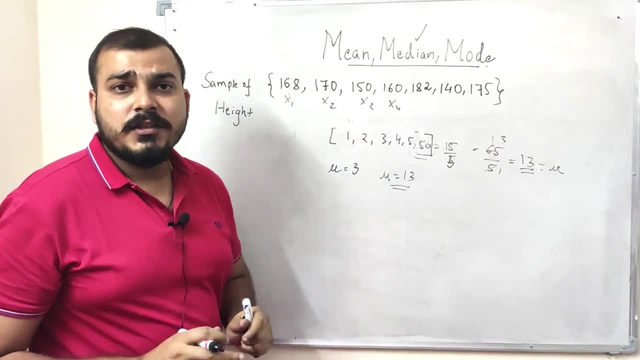 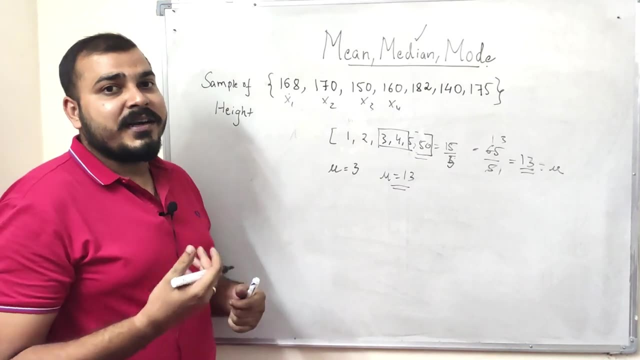 make the numbers in sorted order. Now, currently my number is basically in sorted order. Then what I do is that I will just take the central number. Now how do I decide which is the central number For even numbers, for even count of numbers? over here I have six numbers. 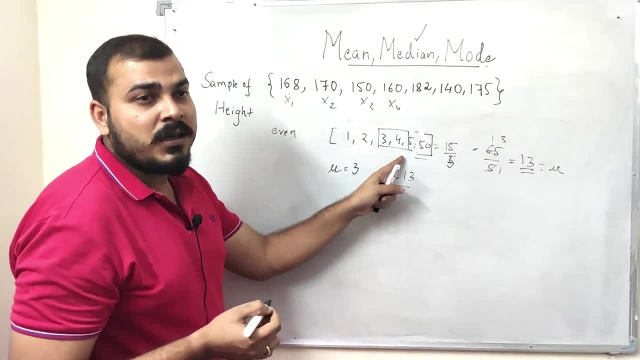 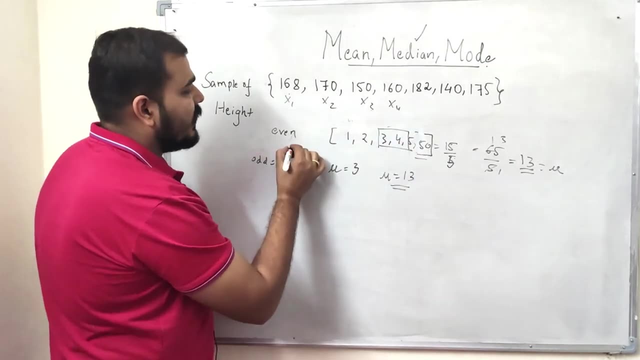 right For even count of numbers. I'll be taking two numbers in the center, Whereas in the case of odd number, this will just be taking the central number. Okay, Now see, if I take this two central numbers, this is three plus four, And again I have to do the average because I 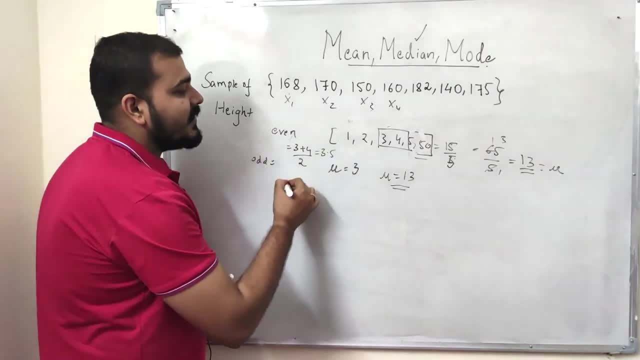 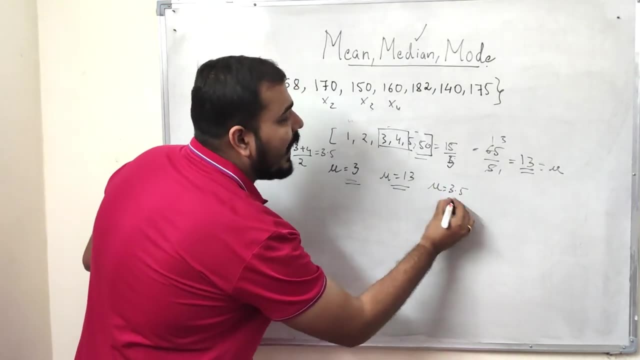 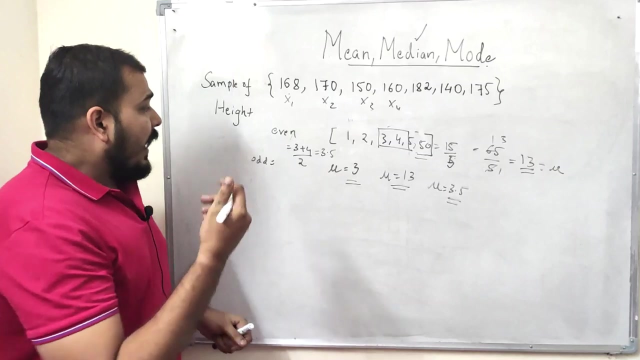 still have two numbers And over here you can see that my central tendency for this, based on mode, will be basically 3.5.. Now you can see that, even though I added an outlier 50, there was a slight difference in the mean Okay With the help of median Okay And similarly. 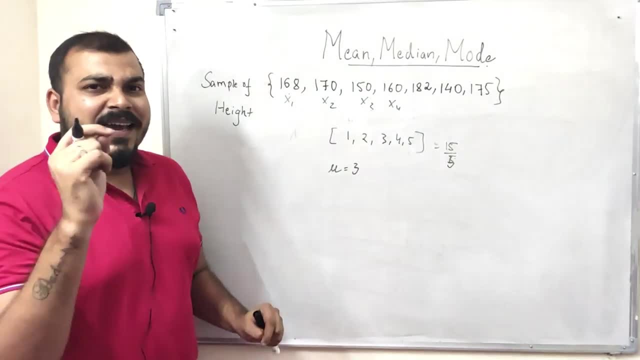 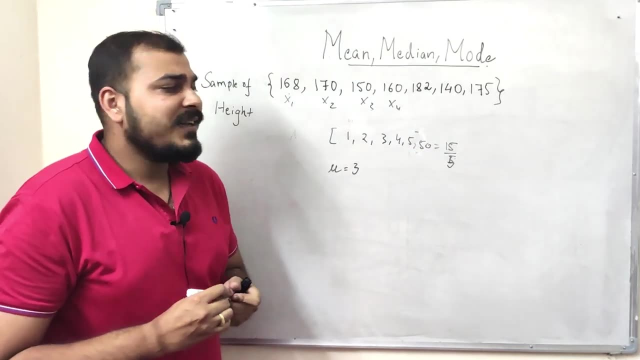 it will be 15.. 15 by 5 is nothing but 3.. Now guess, just understand if I add an outlier like 50. Okay, This outlier basically specifies that this number will be a huge number. It will not be similar to. 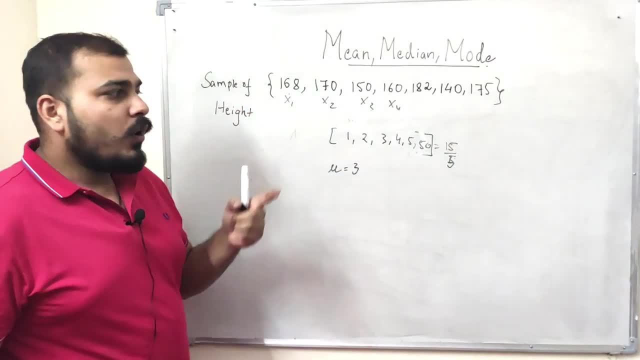 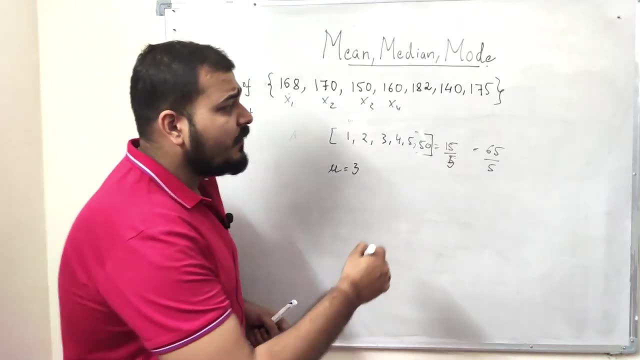 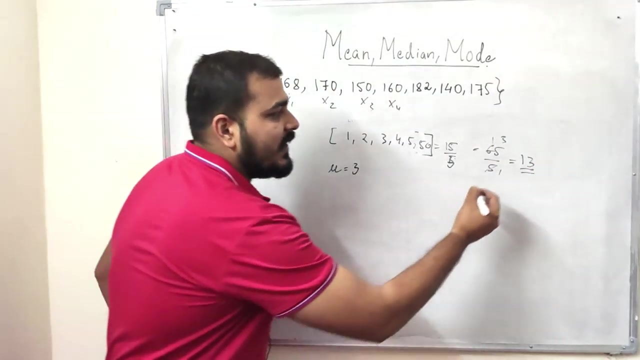 this particular distribution. So suppose I have added 50. Now what will happen is that if I add this up, the total value will be 65 divided by 5.. Right Now, if I try to see how much this is, five ones are three, So 13 is my value. that I'm basically getting Now understand, guys, this? 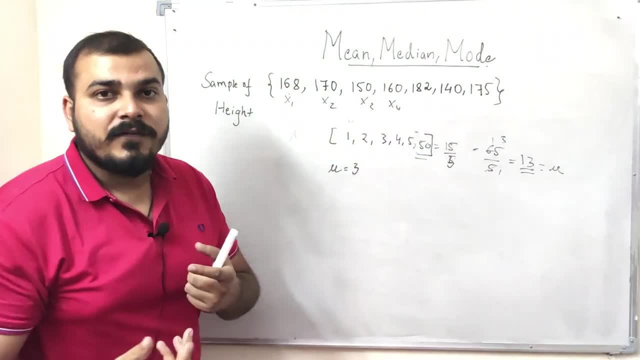 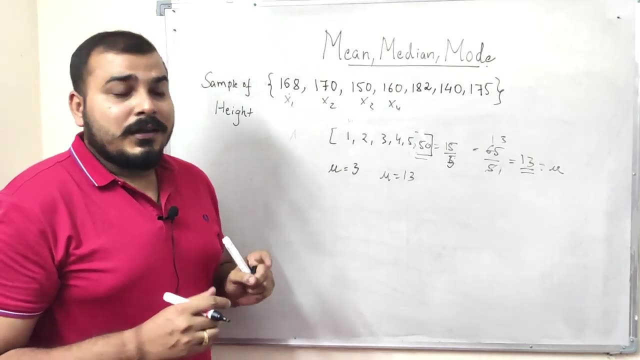 is my new mean after I added an outlier 50. Now you just see the difference of an outlier- Sorry, difference of the mean, because I have added just an outlier. Now this basically represents a complete different format of the distribution And this is very, very harmful for doing any. 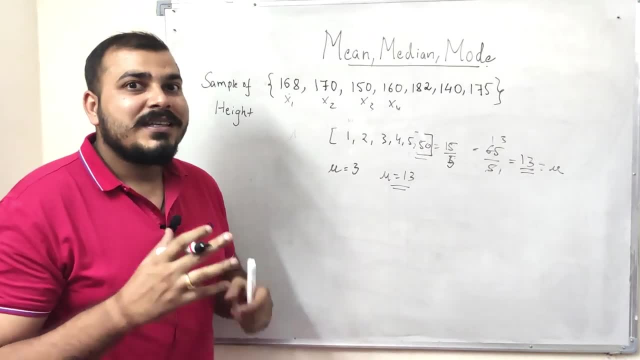 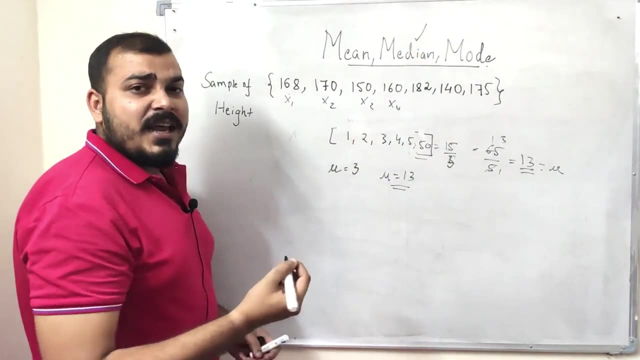 statistical analysis. So in this case, if I want to find out the central tendency, the measure of the central tendency, I can basically use median. Now, how do I use median for median? The first thing is that I have to make the numbers in sorted order. Currently, my number is basically in sorted 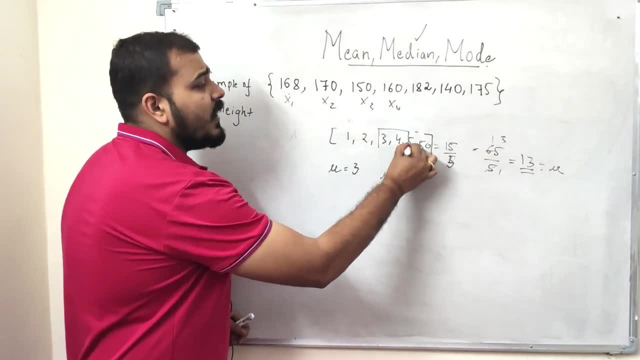 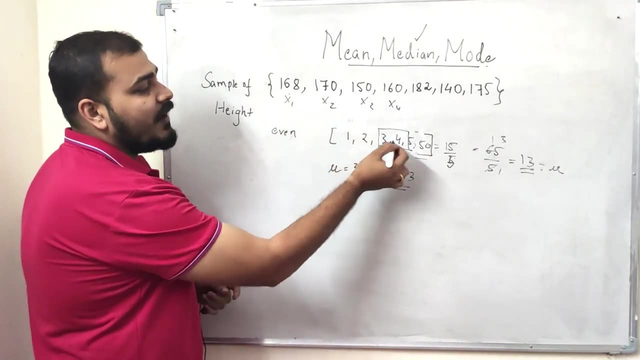 order. Then what do I do? is that, if I will just take the central Number, Now how do I decide which is the central number for even numbers, for even count of numbers? over here I have six numbers Right For even count of numbers. I'll be taking two numbers in. 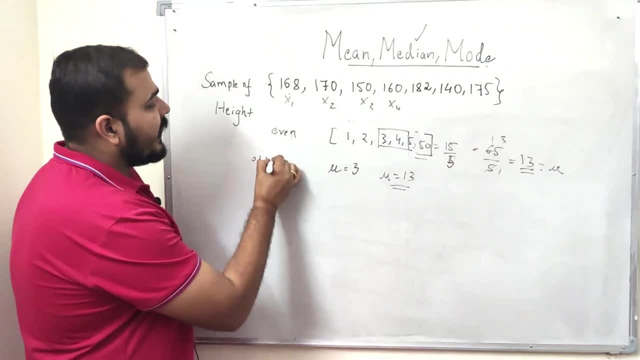 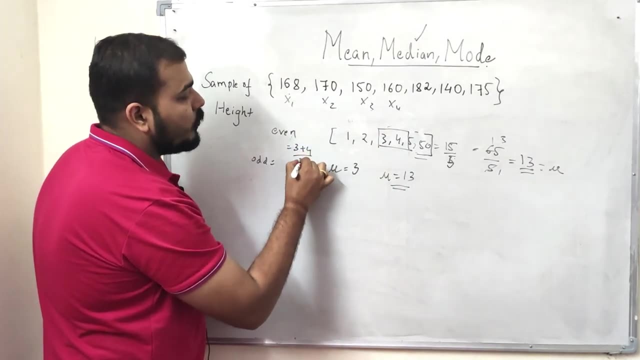 the center, whereas in the case of odd number this will just be taking the central number. OK, Now see if I take this two central numbers, this is three plus four, And again I have to do the average because I still have two numbers. and over here you can see that my central tendency. 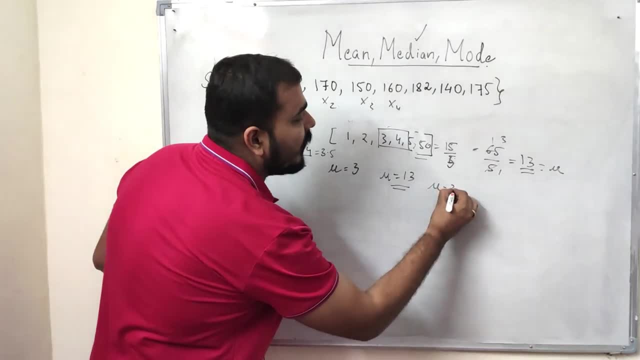 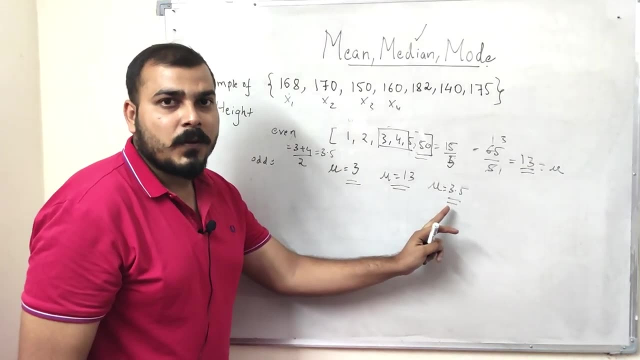 for this, based on mode, will be basically three point five. Now you can see that, even though I added an outlier 50, there was a slight difference in the mean OK, With the help of median OK, And similarly. if I have odd, I just have to select one number which. 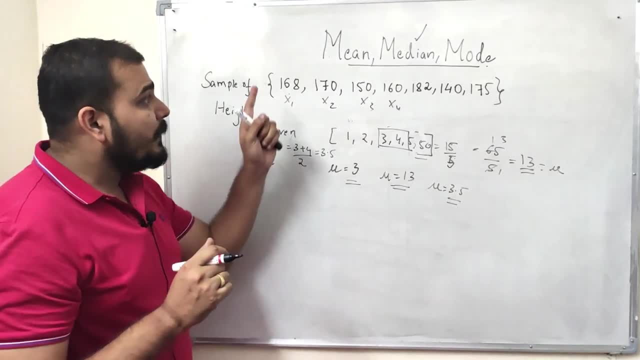 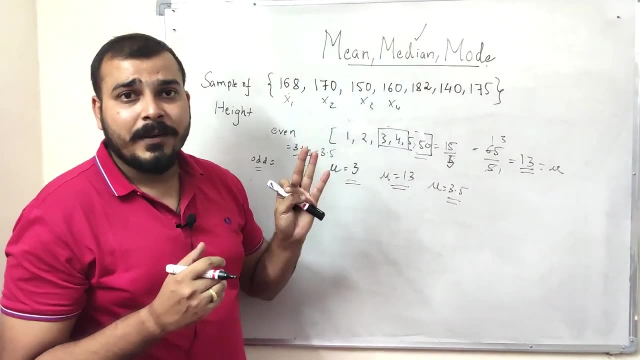 is basically present in the center. OK, So this was all about median And you have understood the importance, because to just lessen the impact of an outlier, we are basically using median And similarly we can also use mode. Mode basically find out the maximum number of frequent numbers in. 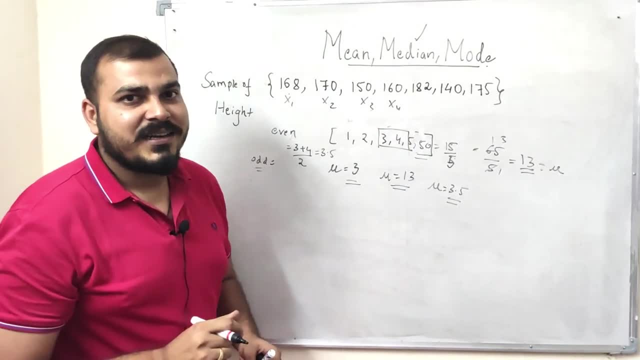 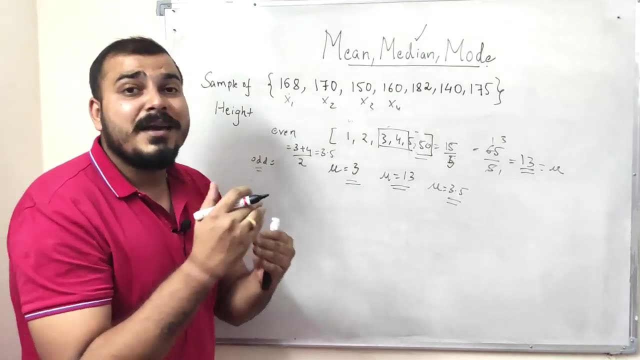 if I have odd, I just have to select one number which is basically present in the center. Okay, So this was all about median And you have understood the importance, because to just lessen the impact of an outlier, we are basically using median And similarly we can also use mode Mode. 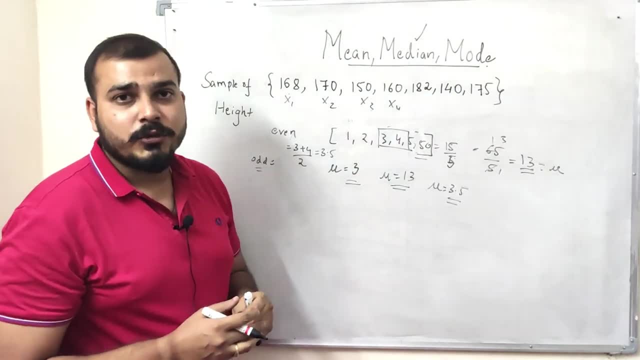 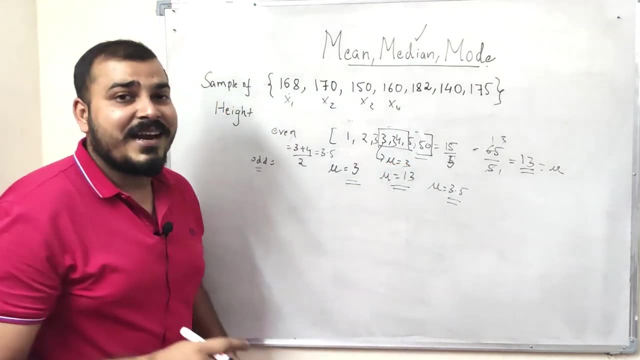 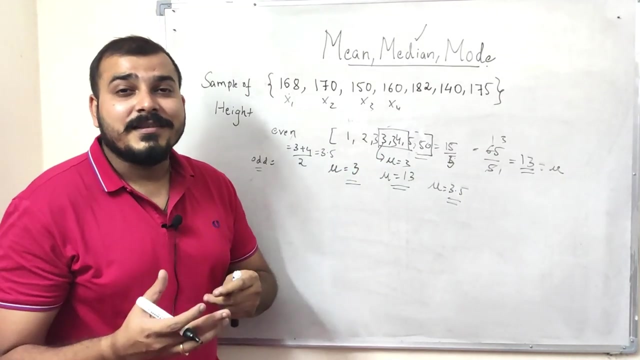 is basically a way to find out the maximum number of frequent numbers in this particular distribution. Suppose my frequent number is three, repeated many number of times. So this will be considered as my mean or my central measure of values. Okay, So this will be basically my value. 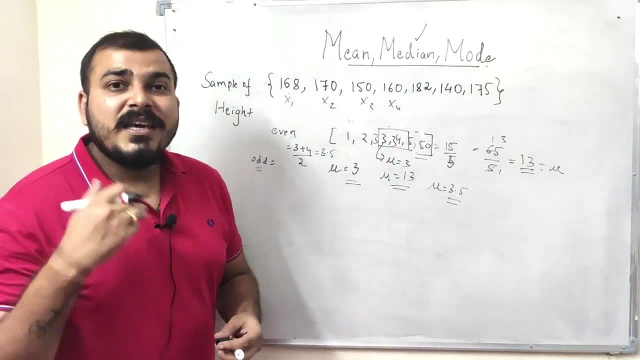 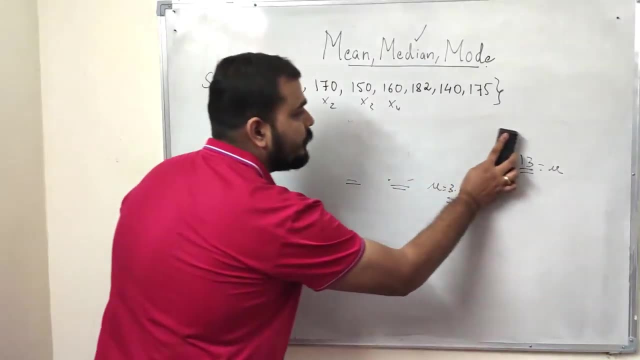 of central tendency. So this was all about median and mode. Let me give you a very good example how this is basically used. So for this I'm just going to rub this and let me just give you a very good example. So let's say that in most of our data set in machine learning we have seen a feature which is called 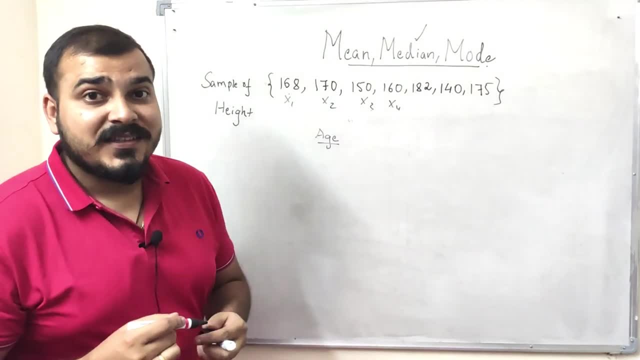 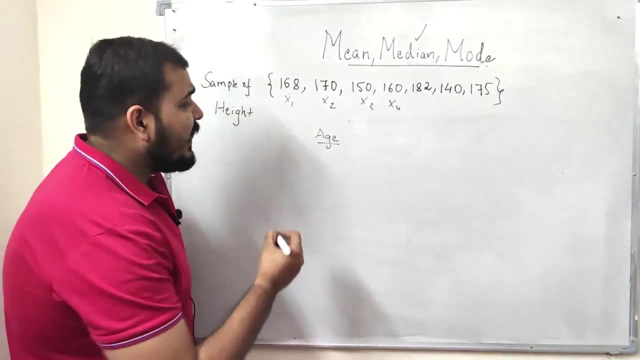 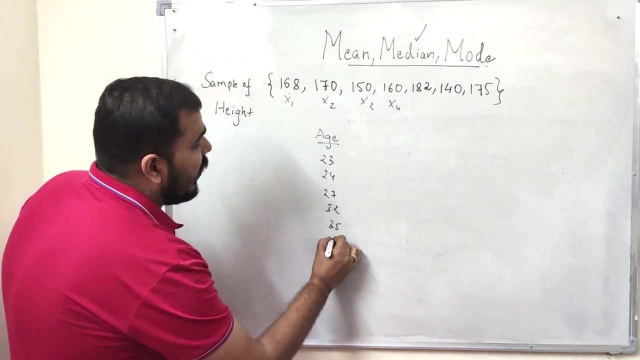 as age. I hope many of them have seen, because in many of the data set when you're doing various machine learning problem statement, you'll have this particular value. Now, when I take age, suppose I have different different days like 23,, 24,, 27,, 32,, 35, and 21.. And suppose I have some 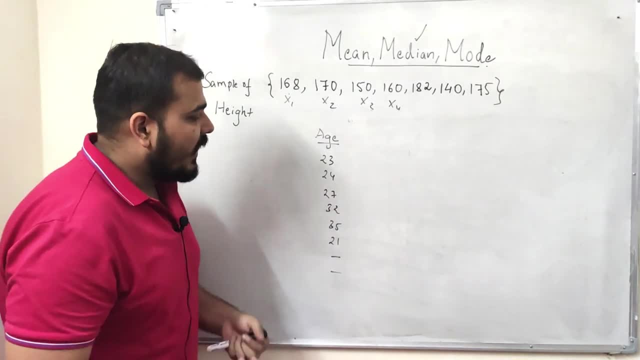 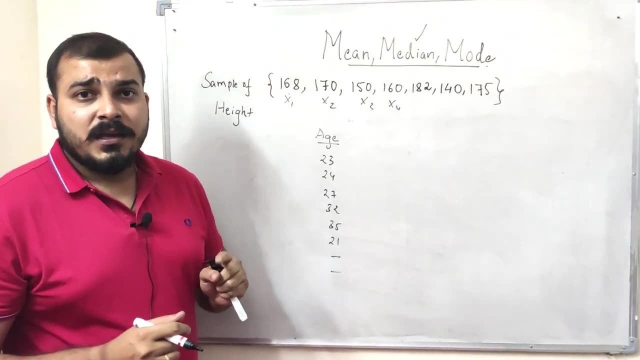 blank values right Now. in this case, understand that the one way. while I'm solving this in data engineering, the first step is basically to handle the missing values. Now, if I want to handle this missing values, there are two ways. Either I can drop this records, But just understand that. if 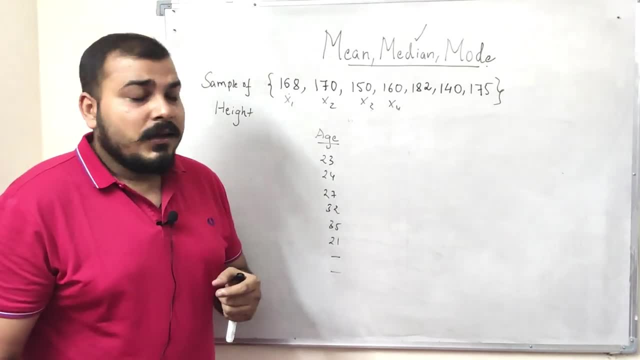 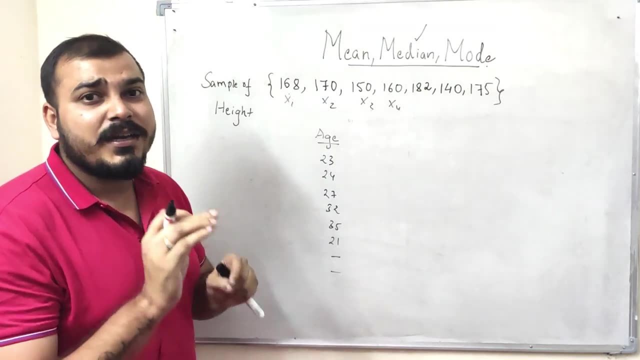 I'm dropping the records, I'm basically losing some information, right? So what we do is that we try to handle this: missing values- And here I'm considering that age is completely independent. it is not dependent on any other feature, right? In that case, what I can do is that I can basically 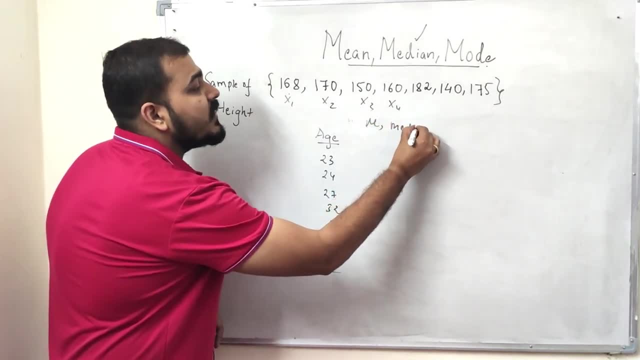 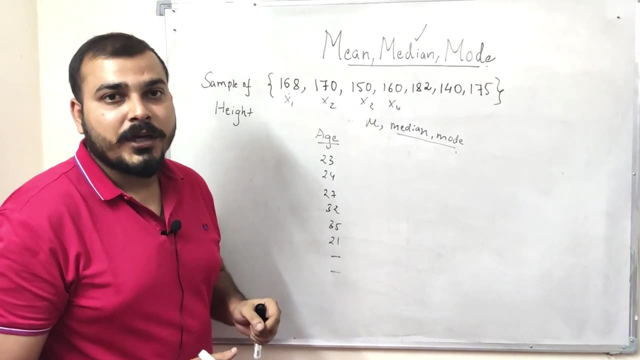 use mean, or I can basically use median, or I basically can use mode. Now, these two will be used only if there are, there is some many outliers present in this age distribution. Otherwise, I'd prefer using mean And then, by calculating the mean, I'll try to. 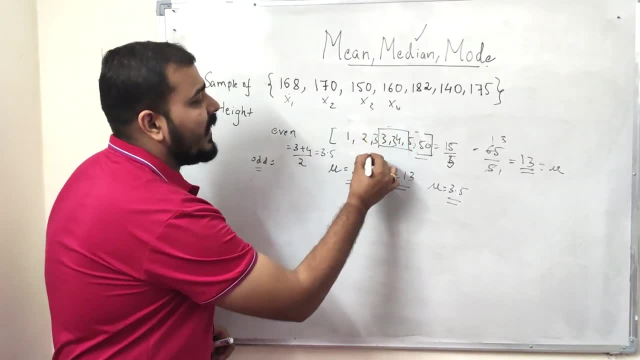 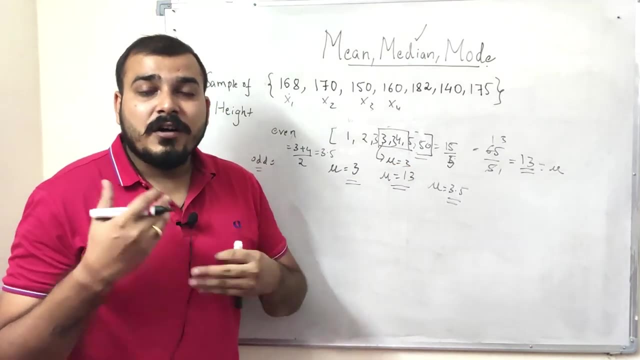 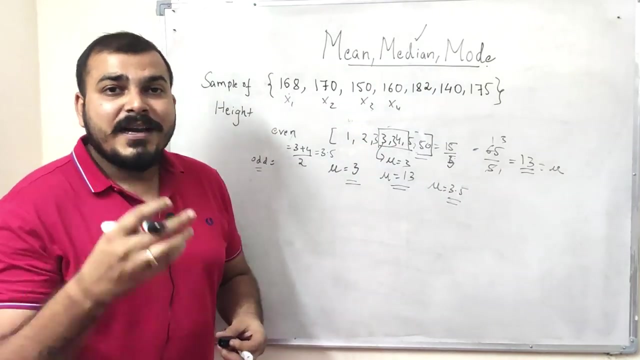 the distribution Suppose my frequent number is 3, repeated many number of times. So this will be considered as my mean or my central measure of values. OK, So this will be basically my value of central tendency. So this was all about median and mode. Let me give you a very good example how. 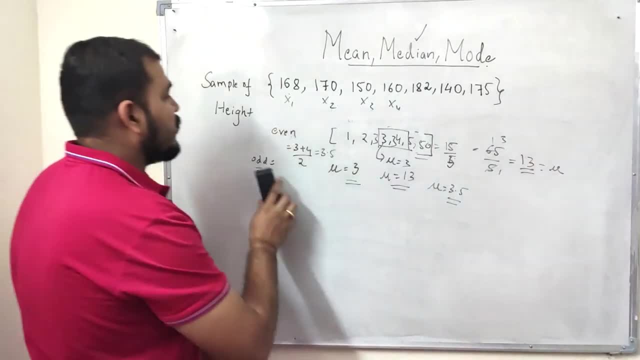 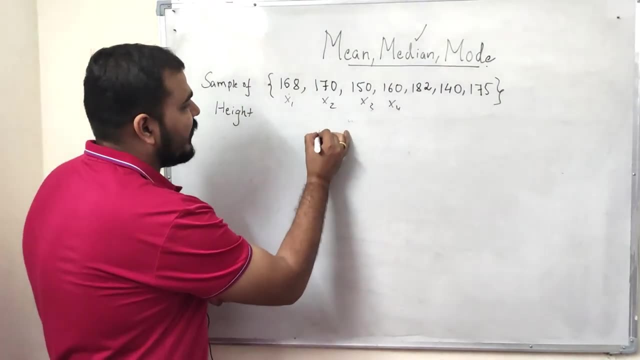 this is basically used. So for this I'm just going to rub this and let me just give you a very good example. Now you know that in most of our data set in machine learning we have seen a feature which called as age. I hope many of them have seen, because in many of the data set 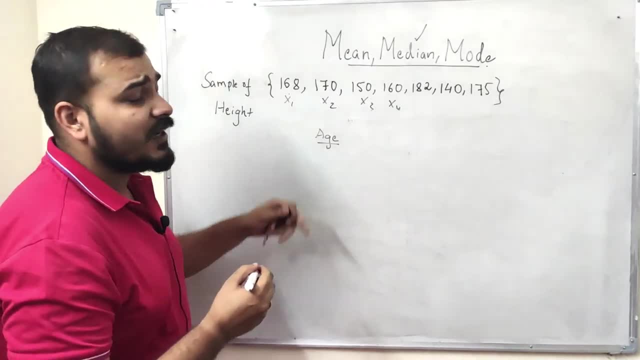 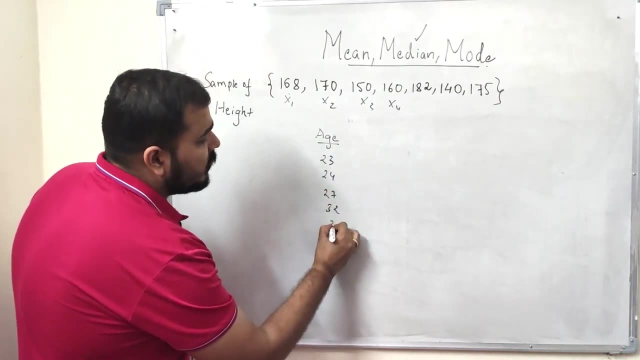 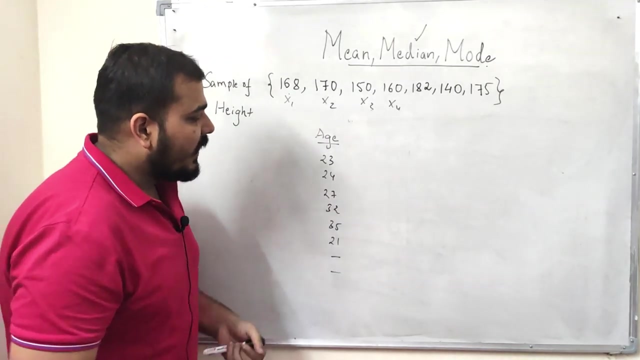 when you are doing various machine learning problem statement, you'll have this particular value. now when I take age. suppose I have different different days, like 23, 24, 27, 32, 35 and 21, and suppose I have some blank values right now. in this case, understand that the one way while I'm solving this in feature. 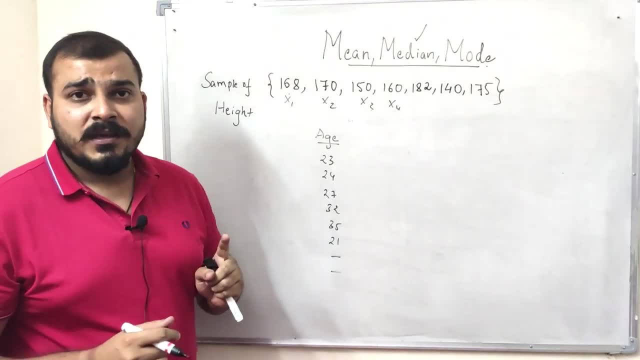 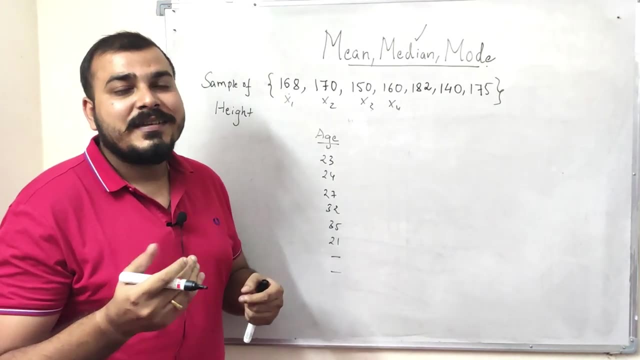 engineering. the first step is basically to handle the missing values. now, if I want to handle this missing values, there are two ways. either I can drop this records, but just understand that if I'm dropping the records, I'm basically losing some information, right? so what we do is that we try to handle this missing. 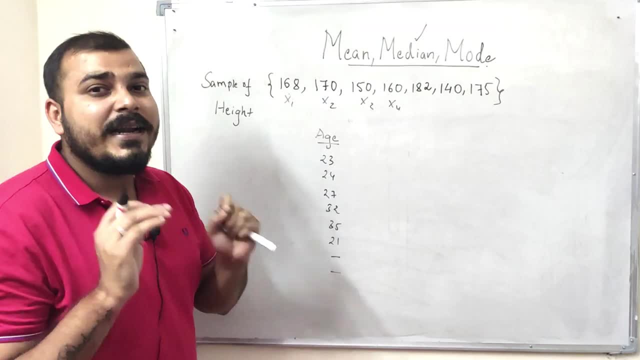 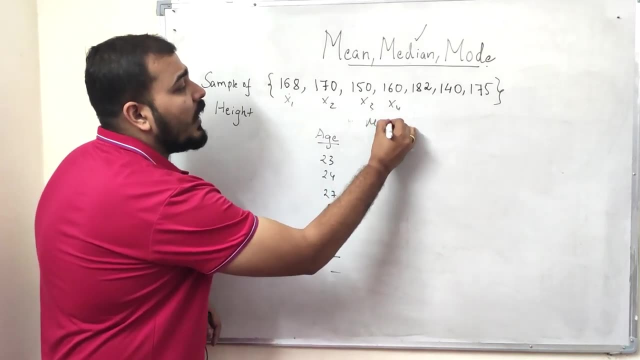 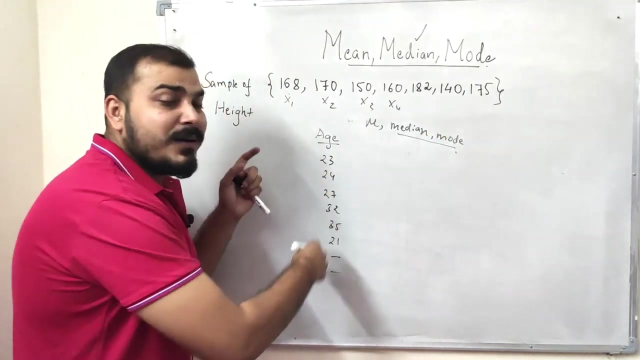 values, and here I'm considering that age is completely independent, it is not dependent on any other feature, right? in that case, what I can do is that I can basically use mean, or I can basically use median, or I basically can use mode. this, too, will be used only if there are there is some many outliers present in 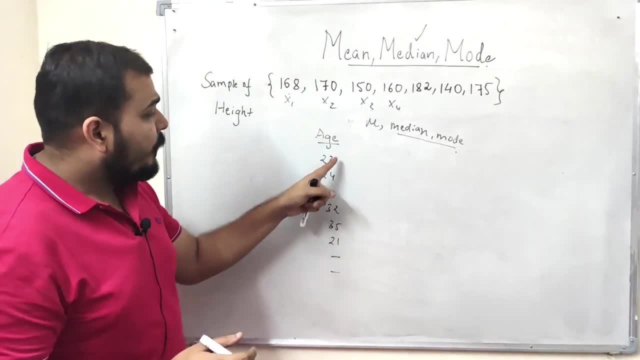 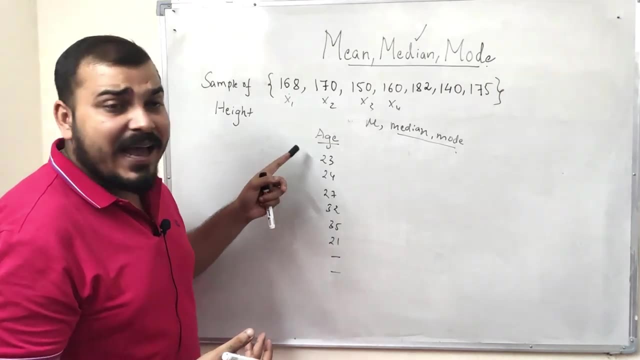 this age distribution. otherwise, I'll prefer using mean and then, by calculating the mean, I'll try to replace in this blank values, and that is how it has to be done. okay, and similarly, if I have a lot of outliers, I can basically use median and mode, and I'll be showing you more examples as we go ahead in the. 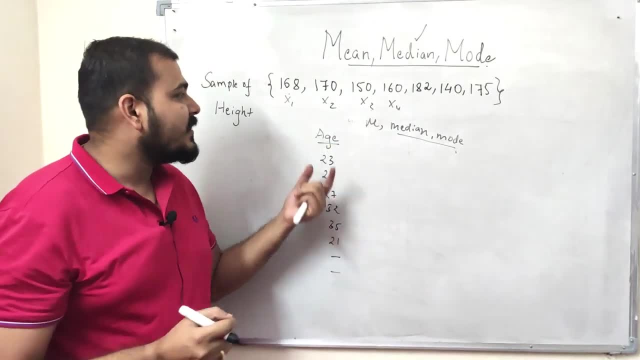 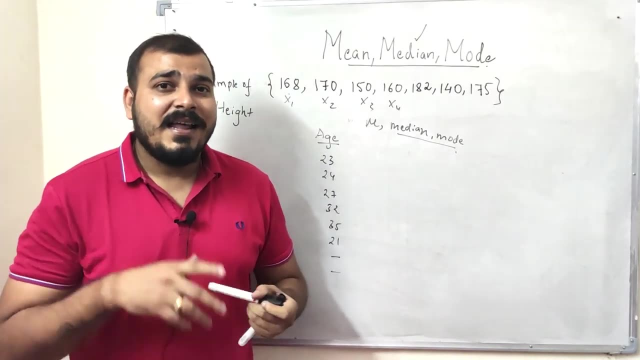 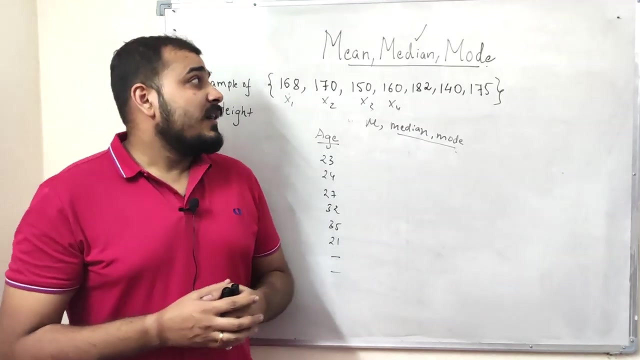 future, but just understand with respect to one data set, and here I've given an example of age. so this was all about this videos, guys. in my next video I'm going to explain you about value distribution and I'll see you in the next video. so I hope you like this particular video and, guys, I'm going to complete this. 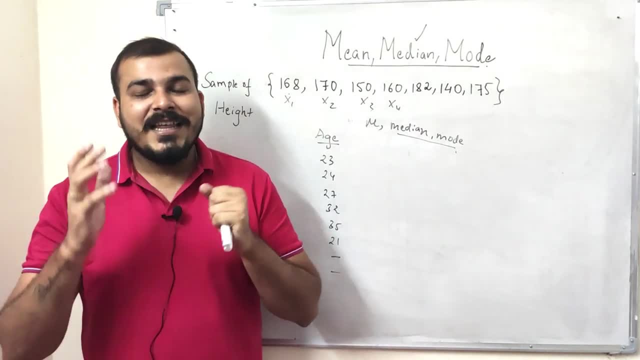 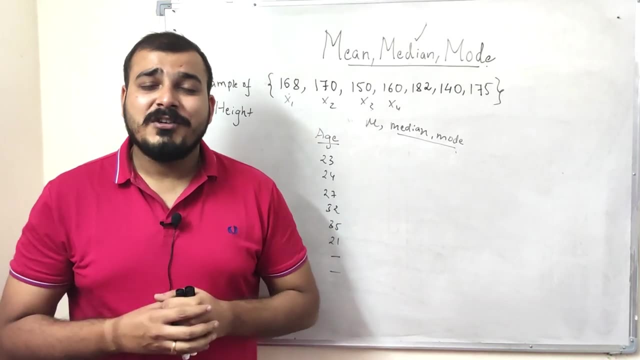 playlist within two weeks. so make sure you watch these videos so that you gain the knowledge and how you can basically apply in machine learning. so this is all about this videos. I'll see you all in the next video. thank you one and all. please do subscribe the channel if you have not already subscribed. till then,